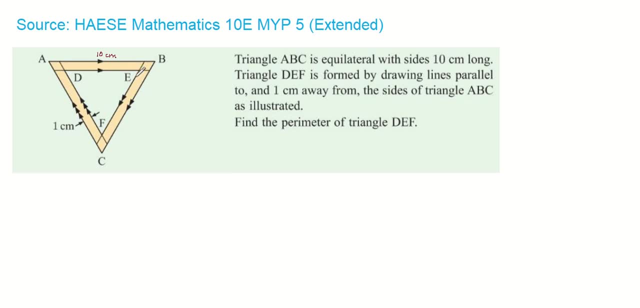 Triangle DEF is formed by drawing lines parallel to and 1 centimeter away from the sides of triangle ABC, as illustrated. Find the perimeter of triangle DEF. okay, Let me just magnify this so we can see it better. So AB is 10 centimeters. 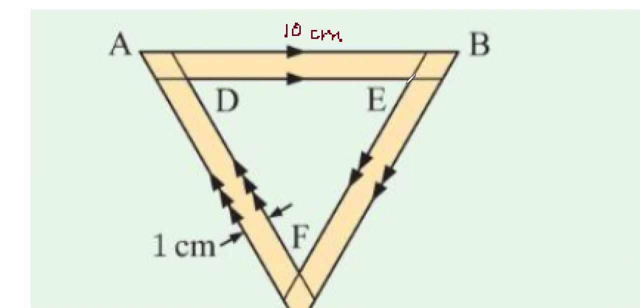 What is DE? If we know DE, then DE is also So equal to EF because they are equilateral. okay, Those two triangles are equilateral, okay. So what are the other clues mentioned here? This thickness here, or the distance between these two parallel lines, is 1 centimeter, okay. 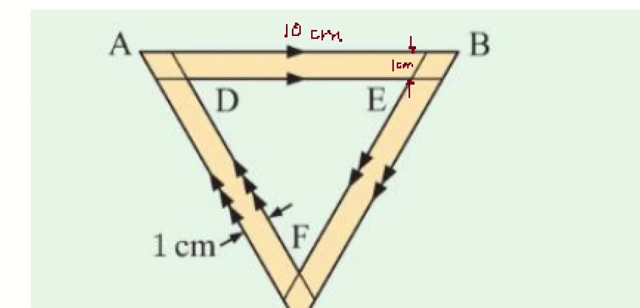 Actually, we can form a right triangle here by drawing. Let's see, Let me see, okay, By drawing this, which is 1 centimeter, this and this line That actually bisects that corner of point B, okay, 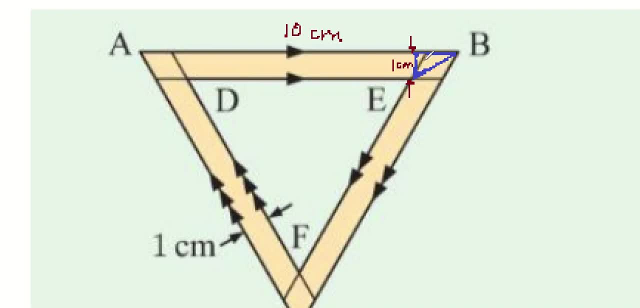 So we have here a right triangle That would be easier for us to solve. So what's unknown, which is D, that side? okay, If we know this side, let's call it X. then this side is also X, okay. 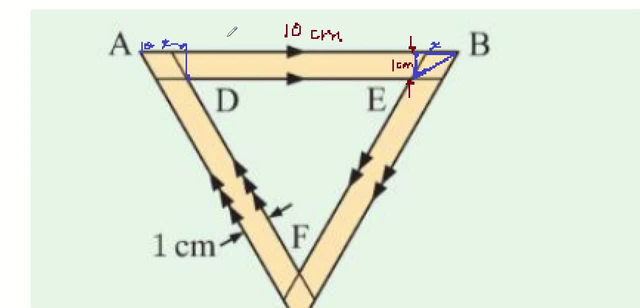 And if we know those two, those Xs, okay, Then we should, We should know the length of DE, okay. What else do we have here? This I would say, since this line bisects this angle, which is 60, because this big triangle here is an equilateral- 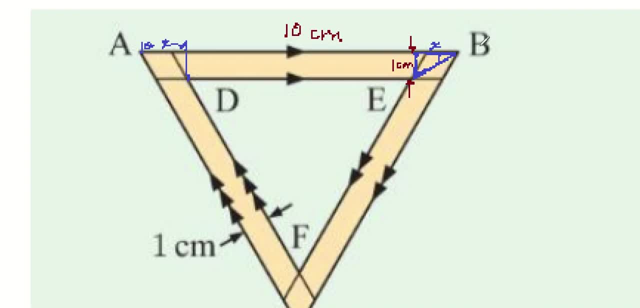 That means the corners of triangles A, B, C is 60. And if we have to bisect that, then this should be 30 degrees. okay, Let me make this one bigger. So what do we have now? We have here 30 degrees and 1 centimeter. 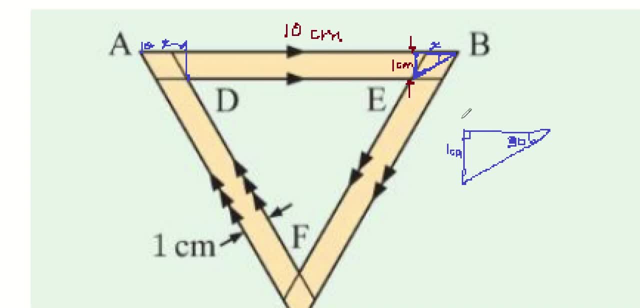 And, of course, this is the right angle because that's, you know, perpendicular to both lines A, B and D. okay, Now we've got two information about this triangle, so that would be easier for us This. 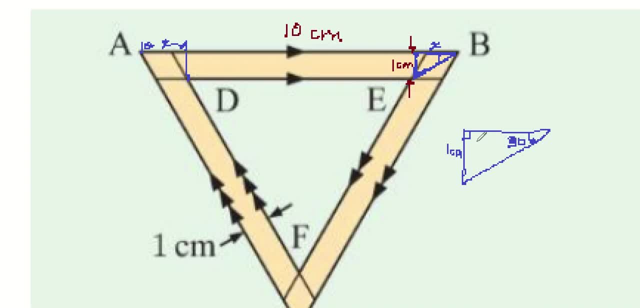 A 30-degree triangle is a very special triangle. Once we know one side, then we know the rest. If this is 1 centimeter, this is 2, and this is square root of 3. If you remember our basic geometry, and then that's it. 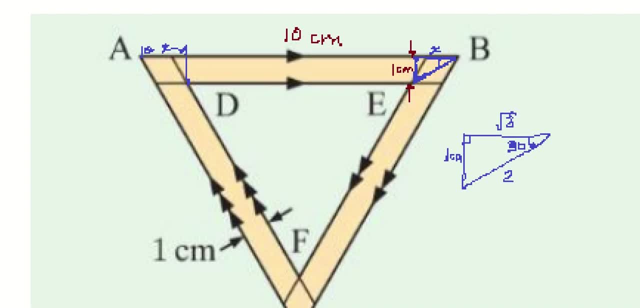 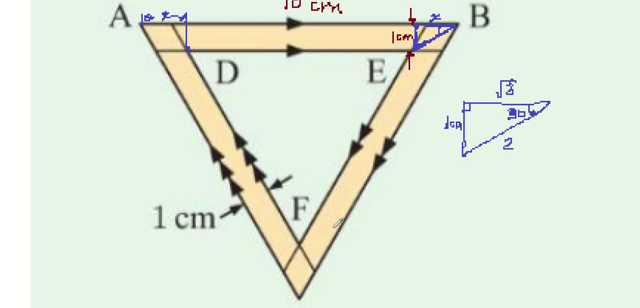 So that's X. X is square root of 3.. Then how do we solve the perimeter of the smaller triangle? So what do we do? So what we do is we have to solve for D, E. D E is now equal to 10 centimeters. 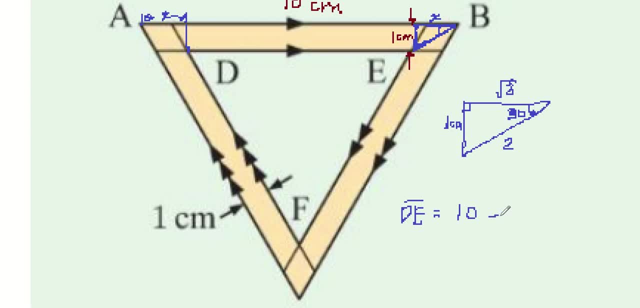 That's A, B minus square root of 3, and there's another square root of 3 there. okay, So that would give us 2 square root of 3.. Okay And well, to get the perimeter we have to add all the sides, EF and DF. 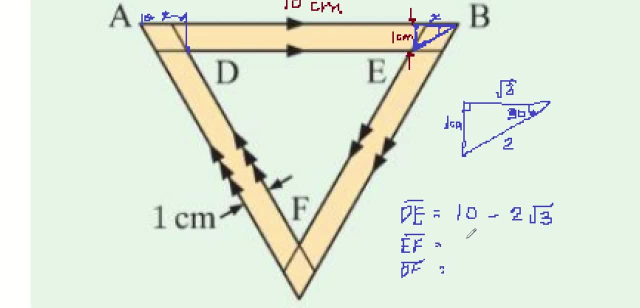 And EF and DF. since they are equilateral triangles, EF is also equal to 10 minus 2 square root of 3, and 10 minus 2 square root of 3.. So if we add, that would be our perimeter. 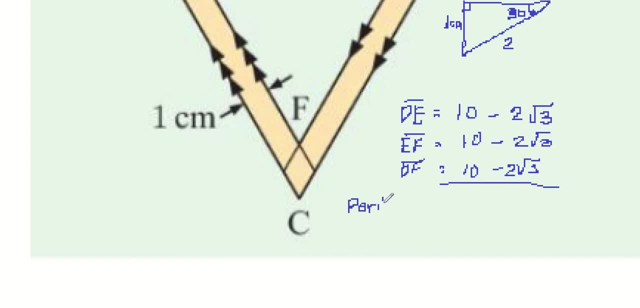 So that would give us: perimeter is equal to 3 times 10 is 30.. 3 times negative: 2 square root of 3 is 6 square root of 3,. okay, But that would be our answer, And well, I can calculate. 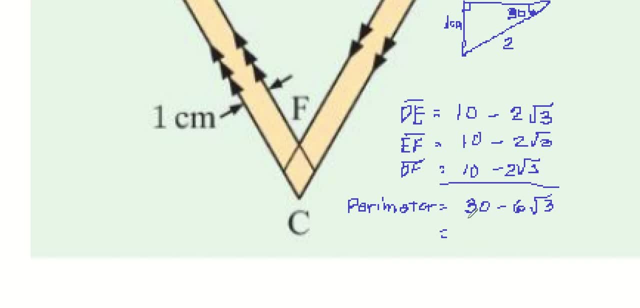 I can calculate this using my calculator. so that would give us 19.6 centimeters. So that's the perimeter. That's our answer.